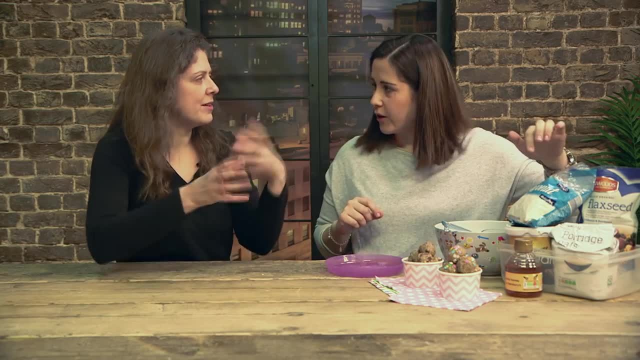 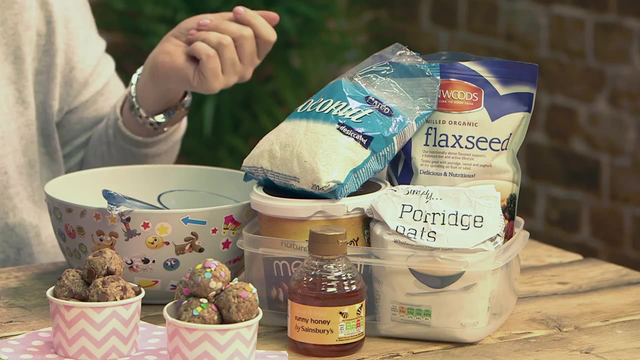 sunflower butter and oats and everything else is extras. Yeah, Everything after that is kind of sneaky nutrition for the kids. Oh, I love sneaky nutrition, Yes. Or a taste: Yeah, Honey as well to taste, to sweeten it up and also helps to bind everything together. I can imagine, yeah, 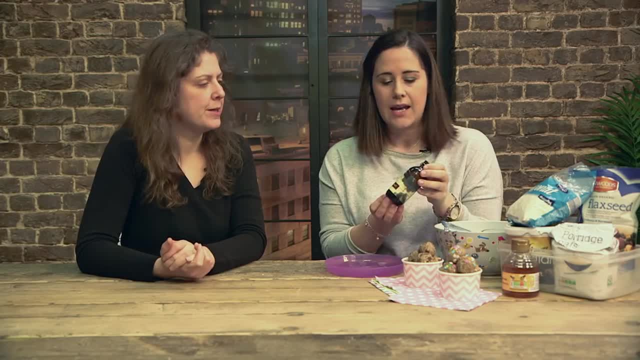 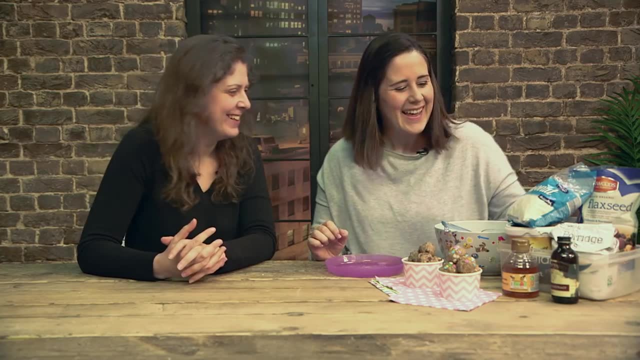 I also like to add a little bit of vanilla extract- Brilliant, yeah, Again, for taste. it just gives it that sweet kind of vanilla taste which is really nice. They smell amazing. And then, finally, any kind of toppings or extra. So today we're going to use these confetti. 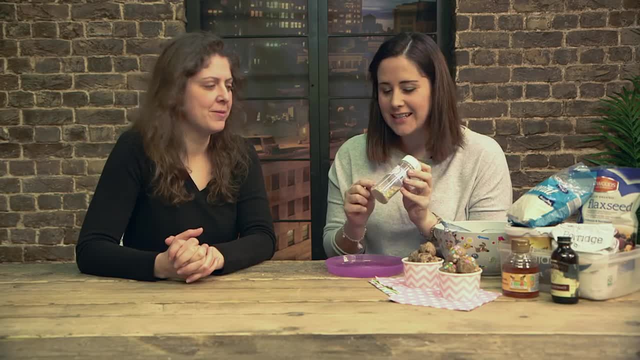 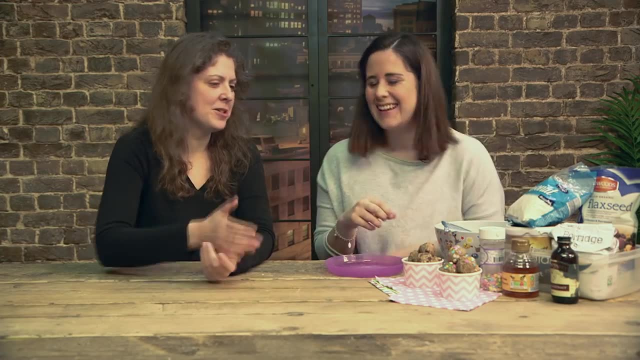 sprinkles, which my kids love, because they see these and they think cake. Yes, exactly, They're obviously not cake, but they think it's cake. Well, it's not cake, to be honest. It's sweet, It's tasty, So you know, And it looks colourful because that is the thing about, Honestly. 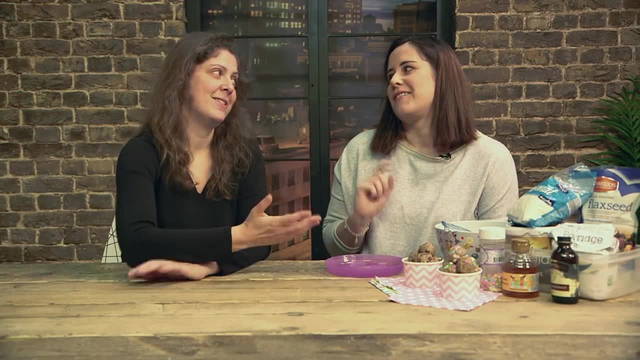 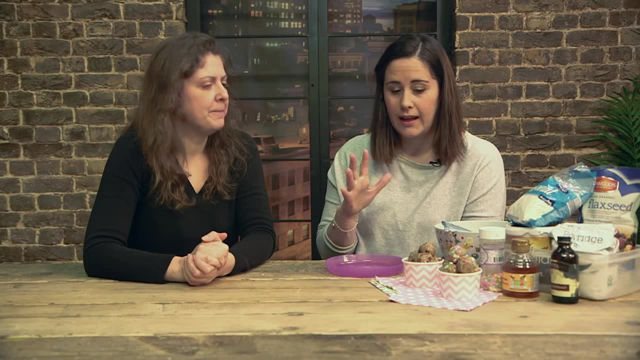 you could roll them in little confetti hearts for Valentine's- Really good idea. Yeah, you could little cookie cutters and shape them. There's so much you can do with this recipe, which is why I love it. Again, you can see the kind of different one that we've made here. We've put chia. 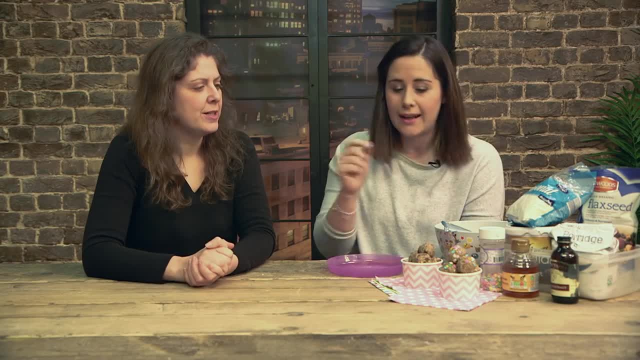 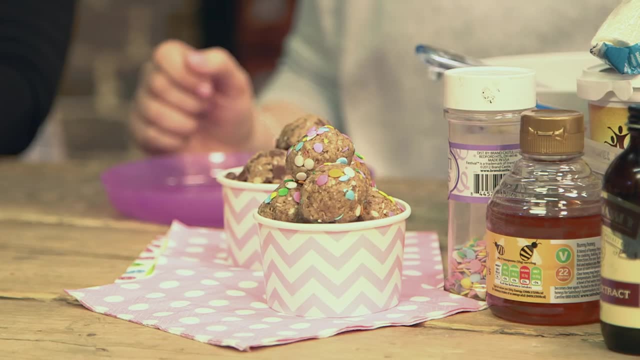 seeds and chocolate chips in this. So again, extra sneaky nutrition. Yes, yes, yes, But then the chocolate is quite. I've been adding some chia seeds to the bread we make just to serve as an extra healthy sneaky. We've got bread maker. obviously I'm not making it from scratch. 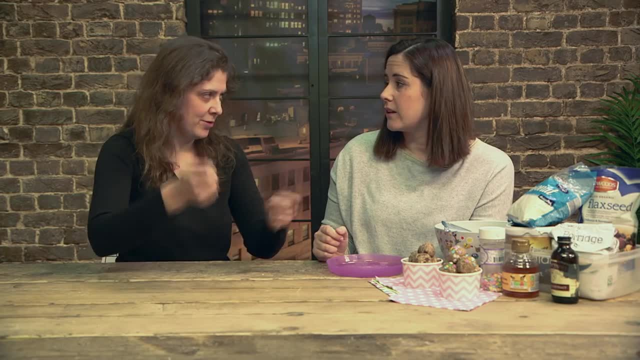 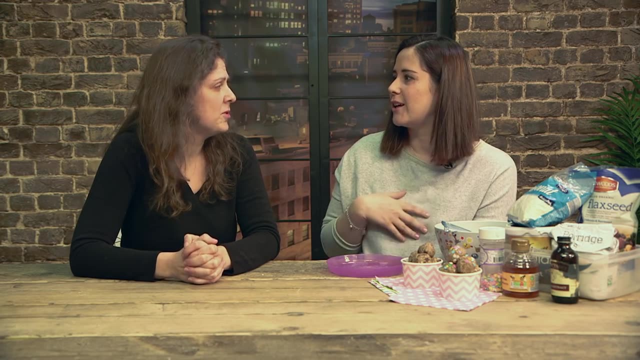 But you know it's the sneaky way to get in some healthy vitamins and minerals and stuff. There's so much. I mean I make chia jam because my kids love jam on toast in the morning, Oh yeah. So I make it with honey and chia seeds- Clever, Which they just Again, they have no idea what's. 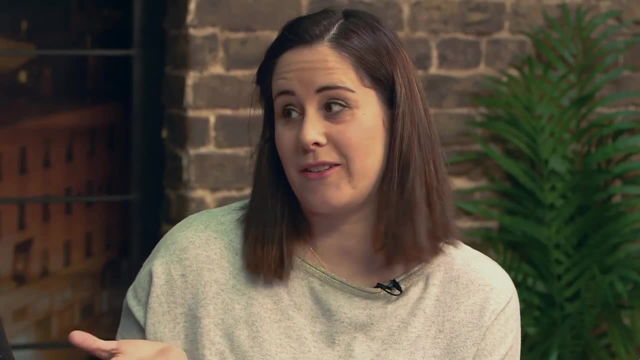 in there. No, it doesn't matter, does it? Smoothies and bread. Never thought of bread. That's a really good idea. Yeah, just as Especially if it's the granary flour, But I guess with white flour. 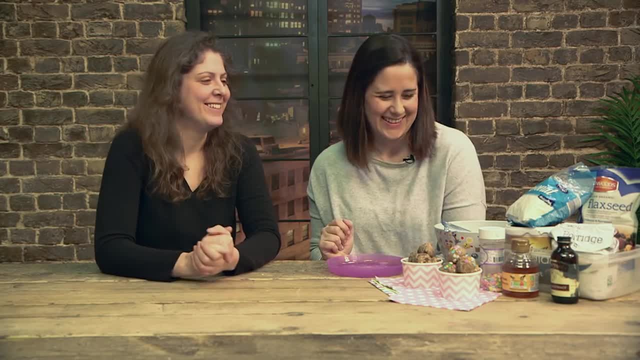 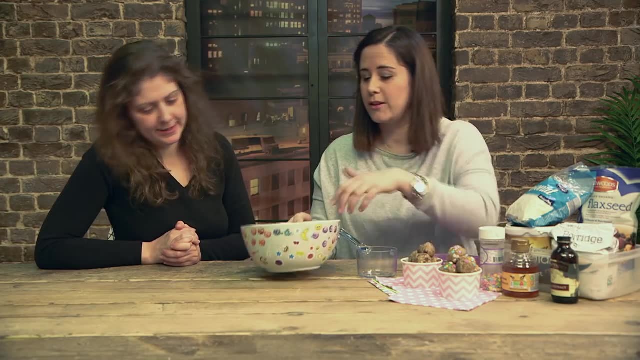 you wouldn't really notice so much. Yeah, Yeah, I love a bit of chia seeds, Great. So let's get started. So that's it. Yeah, So all we need is a bowl, a lovely decorated bowl, My daughter. 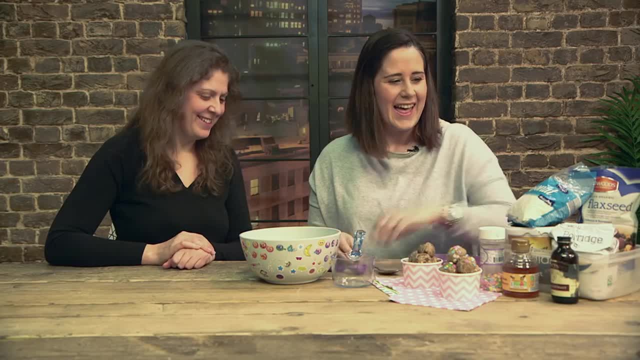 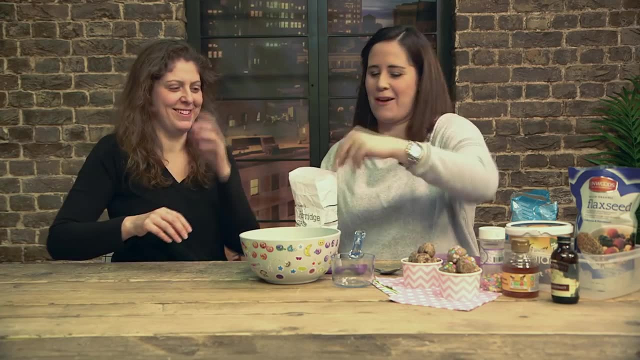 decorated with stickers. Oh, cute And Okay. So do you want to do it? Oh, we'll do it together. Yeah, You can do the messy bit. Okay, You can do the measuring. We might have to do it with the kids. So one cup of oats. 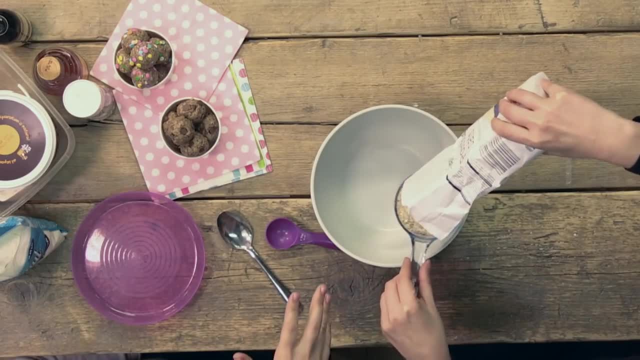 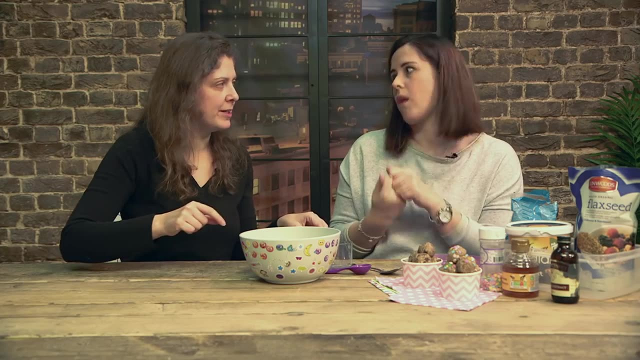 And I always use a cup. So I know that's kind of like American measurements, but even for a lot of That's perfect. For a lot of UK recipes I use cups because it's just easier than- And especially if kids are helping you right? Oh, exactly, I just I don't. I'm too lazy to drag the. 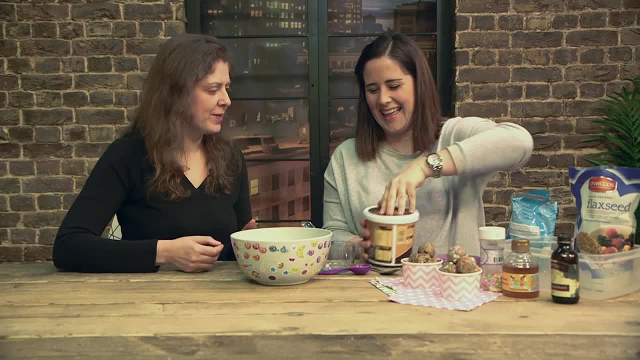 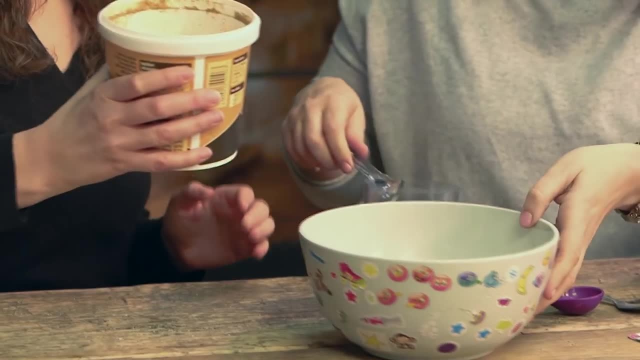 scales out all the time. Not lazy, It's time poor. So it's one cup of oats and then a half a cup of your peanut butter, nut butter or whatever it is that you're using. Oh, that's quite runny actually, That's. 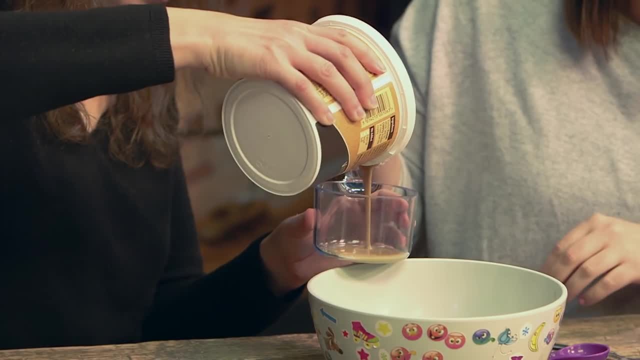 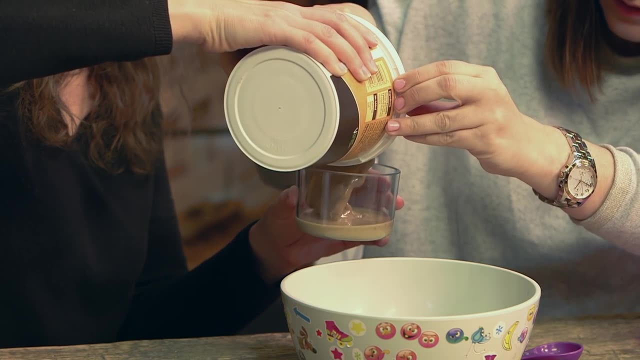 interesting. So half, Yeah, So half of that, Yeah, Oh, this would be fun. Oh, yeah, So you're helping us. I should have probably stirred it, shouldn't I? Sorry, It's okay. Does it matter that we took the liquid out first? 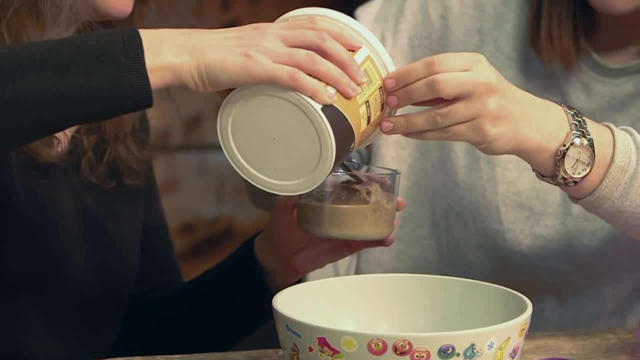 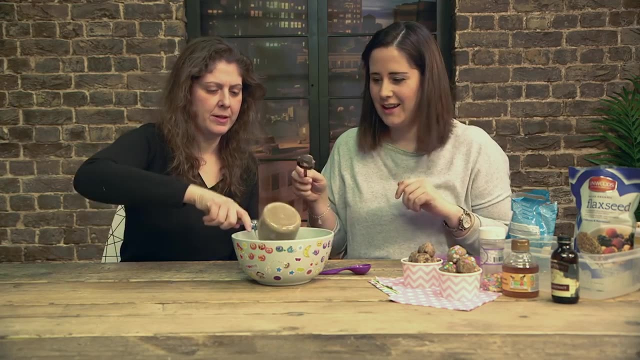 No, I think there's just this, This. It looks about half, doesn't it? This brand of peanut butter. I think it kind of separates because it's supposed to be quite natural. Yes, That's always good. Would you like a tip? Just Yeah, Chuck it straight in Great. 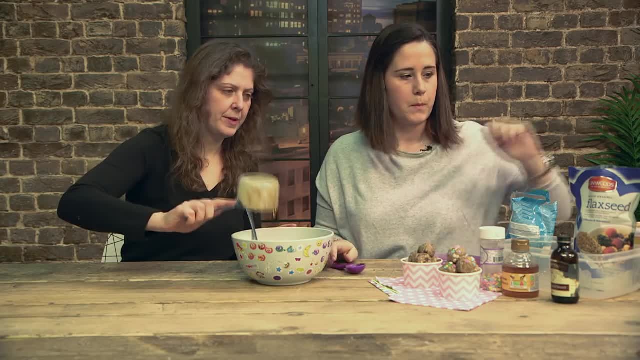 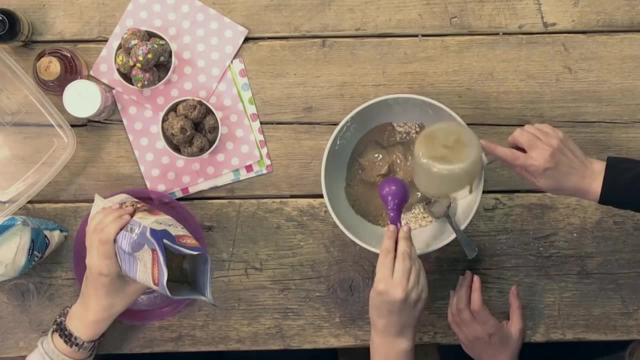 And then we're going on to our smaller measurements. We need a tablespoon. I'll let you do that whilst I drip this. Okay, So we need two tablespoons of the flaxseed Brilliant, Which, again, I put into so many things. Oh, and that's ground. 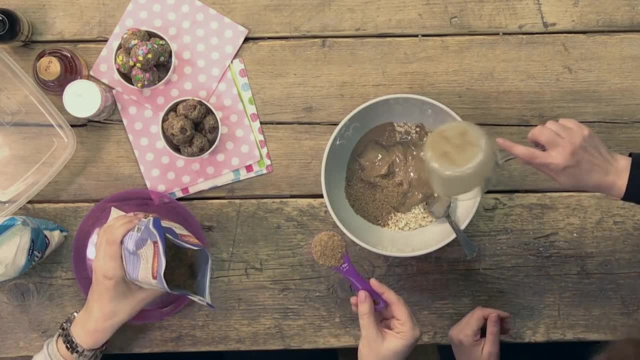 It's ground, Yeah, So the ground flaxseed And it's probably better to digest, is it? It is, Yeah, Apparently, it's a lot easier to digest. And again, it's not bitty, because your kids don't like little bits. Yeah, They like it. No, They like it. 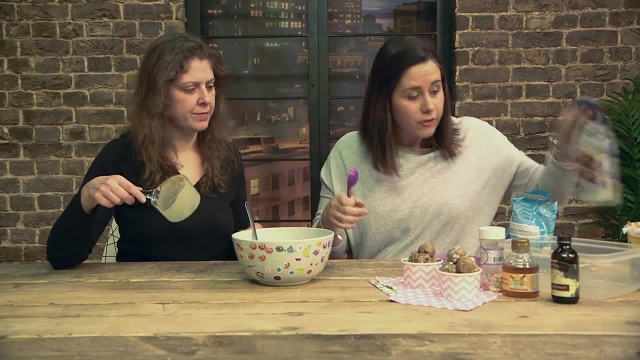 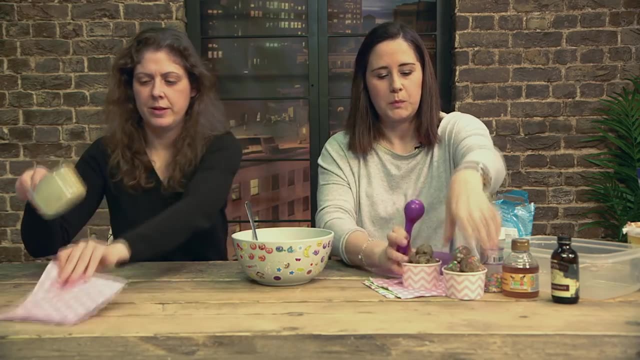 And, yeah, I love this because it's full of fiber, omega-3s, which we know are so important for growing children. What do you need? We're going to roll onto that. Okay, I'll take a napkin. You can take a napkin. There we go, So, yeah, So if you have kids that don't eat fish and you're 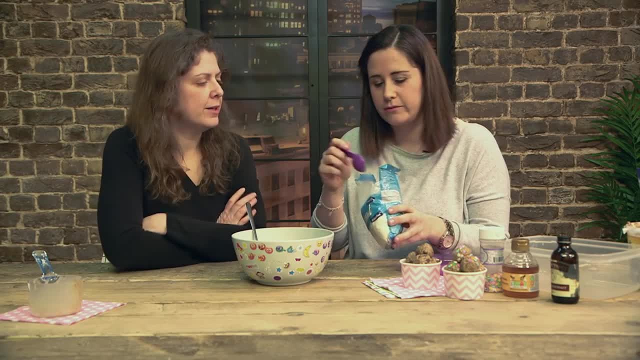 worried about getting omega-3s. flaxseed is a great alternative. Brilliant, Thank you. That's good. Yes, My son doesn't. My daughter does, So it's good for my son. Yeah, Definitely Well. 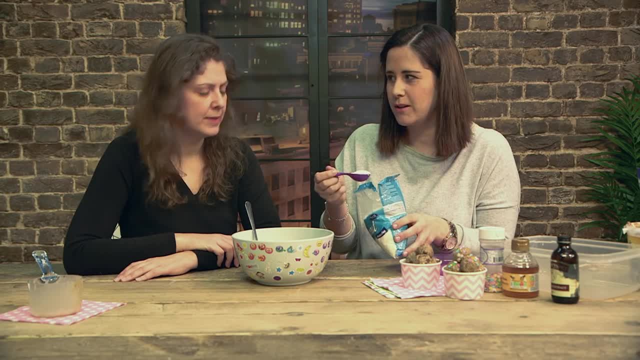 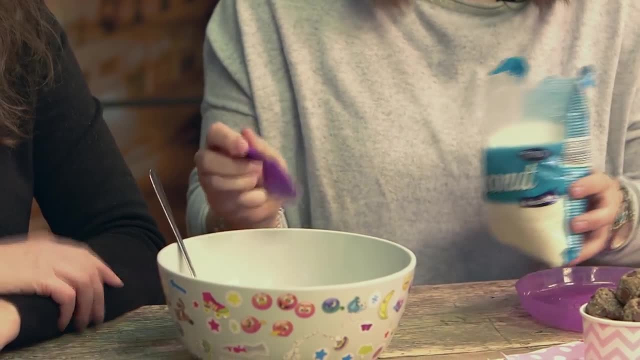 both of them, obviously, It's just. It's one of those foods that can be quite tricky, especially with younger kids. Yeah, Onto the shredded coconut. we're going to need, Yeah, Two tablespoons of this as well. Excellent, Just start stirring once you get there. Yeah, 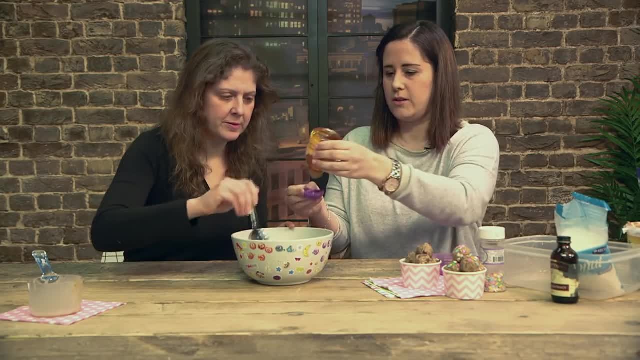 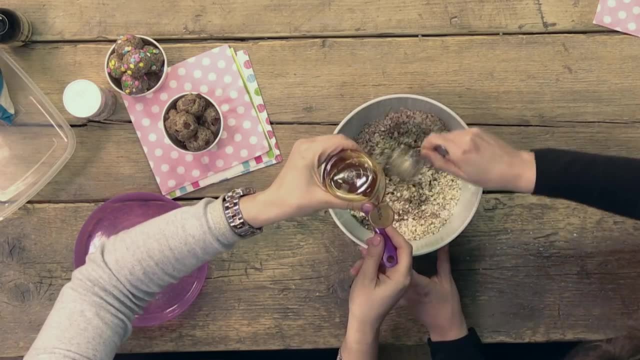 you can stir away. And then finally the honey, another two tablespoons, Okay. So it's not too much, It's not? I mean, considering the amount you make. I usually get about 12 energy bites from this, Okay. So two tablespoons of honey for kind of 12 portions, I think is quite good Yeah. 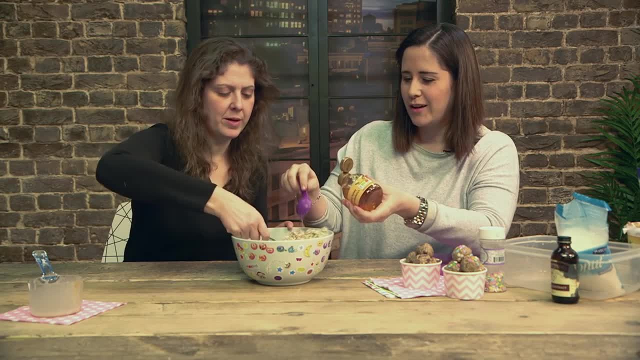 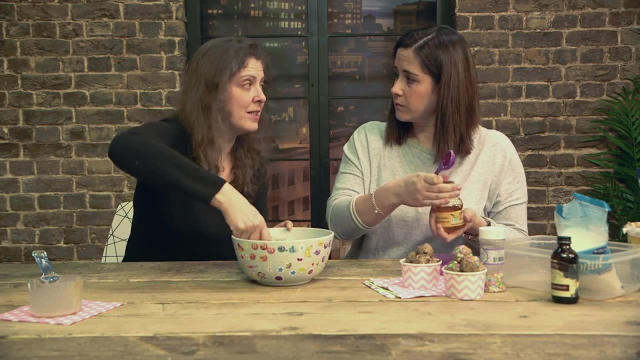 It's an easy recipe to remember as well It is. Yeah, I'm going to so make this with my kids. I'm thinking, even if we use the sunflower butter, I might do these at my son's birthday party with the kids. Yeah, that's good. One of them has got a mild nut allergy, but you know intolerance. 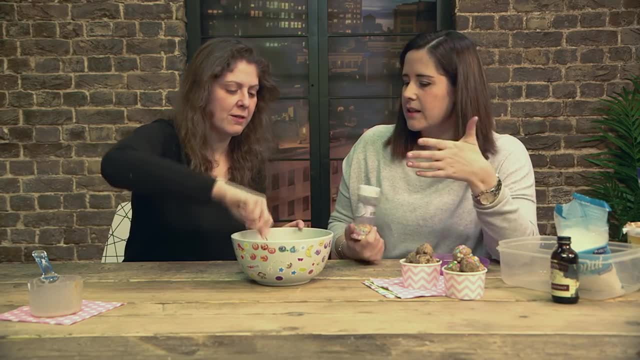 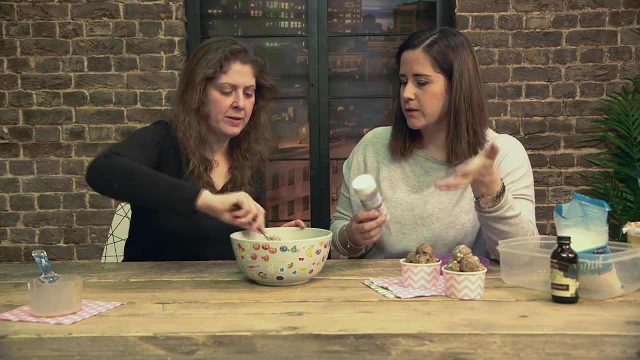 but I still think obviously it's good to go safe And sunflower- if I use that- then that's quite a nice way of, you know, making it really inclusive but tasty, Absolutely, And especially if you want to send them into schools, because so many schools are not free now and it. 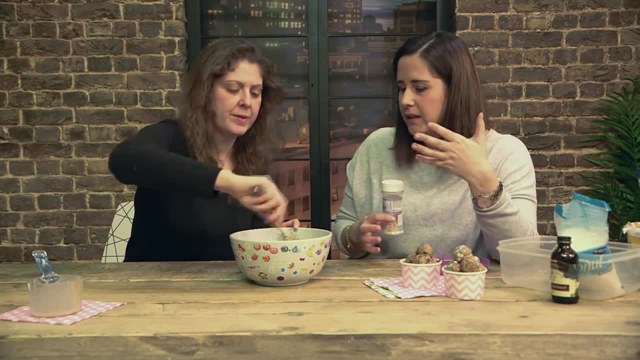 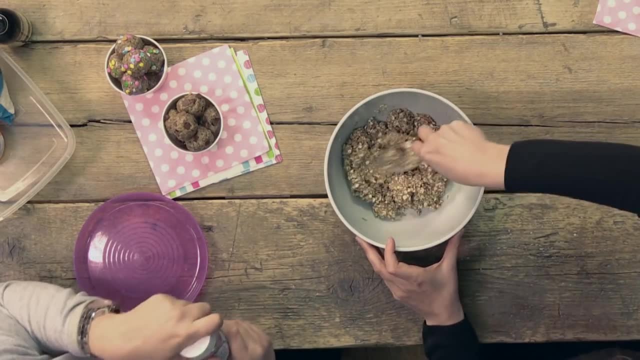 does make kind of healthy treats a little bit tricky. Yes, How's that? So? yeah, Is that good, Maybe a little bit more Sorry. Yes, mom, You can get in there with your hands. I was going to say, would you get your hands in? 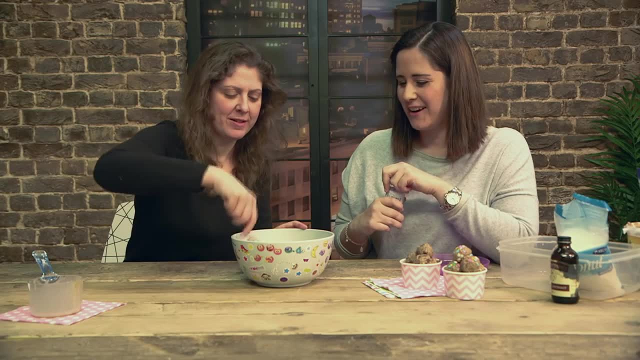 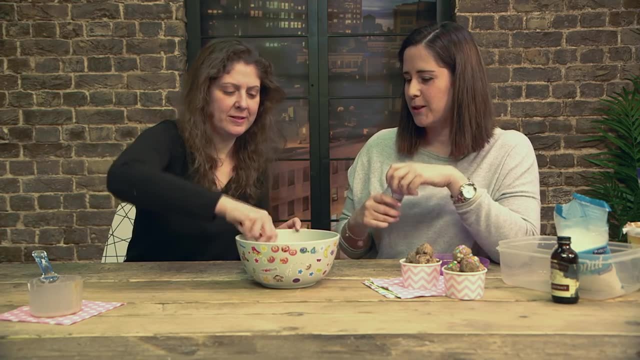 or at home you'd probably with the kids. My kids get straight in there with their hands, but it's fine just to mix up. How old are your kids again? Almost five. Four are going on five and my son is just coming up to two. His birthday is in a couple of weeks. Oh, very busy house then. 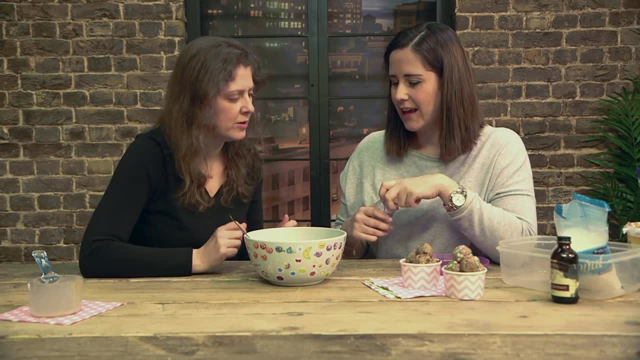 Yeah, Okay, How's that? Is that good enough? I think that's good Enough to roll a couple of balls. We're going to add the sprinkles now. Oh, you add them in now, So we're going to add them. 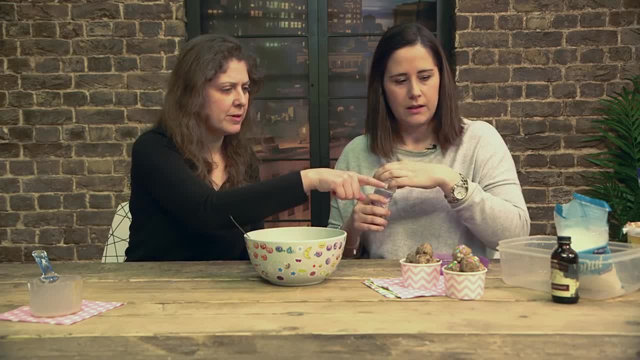 in now and then sprinkle a few more on top as well. Can we do the vanilla? I can't remember. Oh, we didn't do that, Just because you've got it Again. you see, you don't have to, It's made. 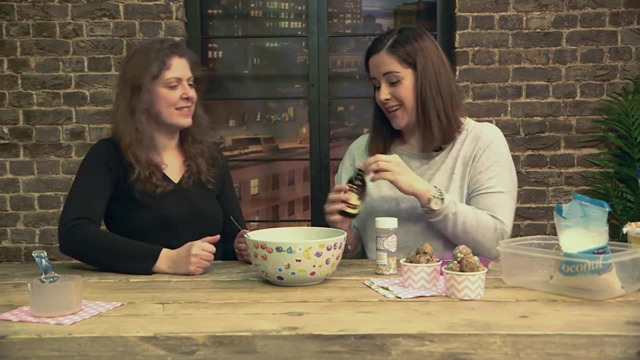 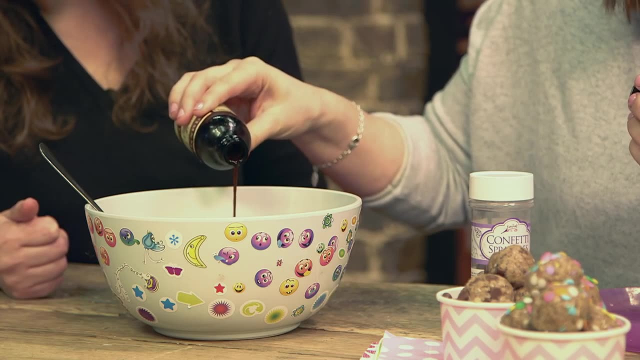 up as you go along, in that sense. So it's not the exact science. Whatever you have in the cupboard, just chuck it in, But as you've got it. So the vanilla, yes, about half a teaspoon. Okay, That's usually enough. I measure this by eye because, again, I'm too lazy to get the spoon. 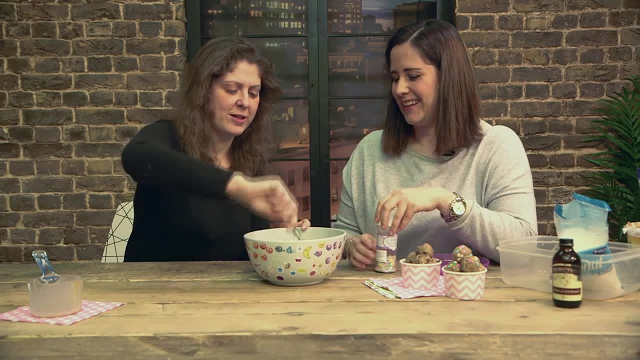 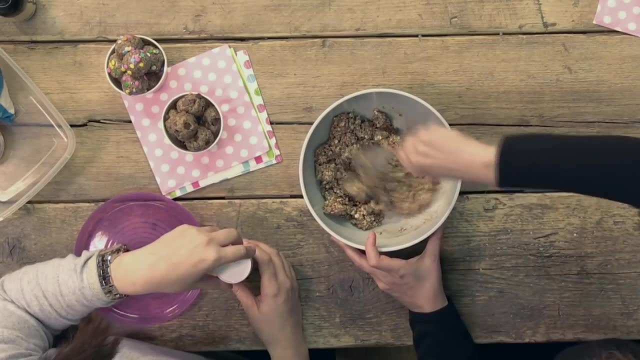 from the drawer. No, it's good. It's not lazy, time-economic, sensitive or whatever. economical. Oh wow, This smells amazing. It does smell good, doesn't it? Yeah, it does smell really good. I think it's a combination. The peanut butter smells good, but then the sweetness from the honey. 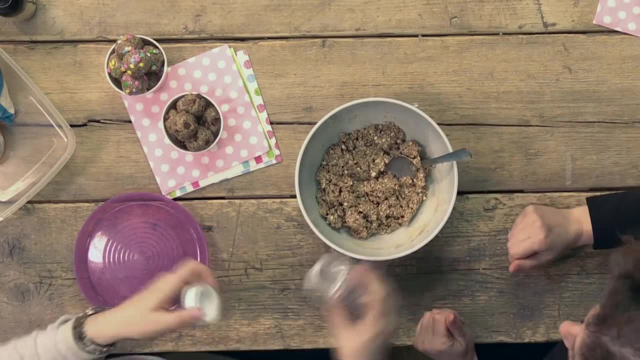 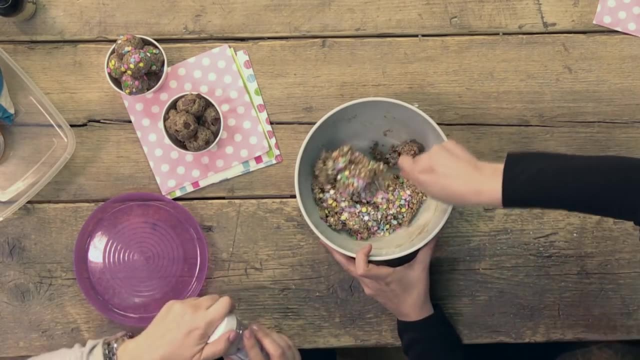 and the vanilla, it really starts to smell good. Now we're going to add the sprinkles. You could just do this by eye. I thought you were going to roll it in afterwards, So it's fun that you've put them in already. Yeah, I put them in just to make sure they go all the way through. So 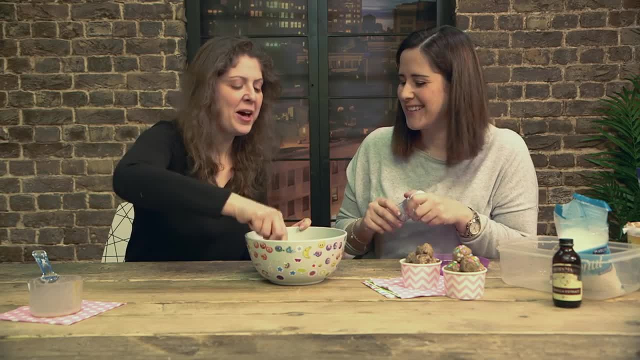 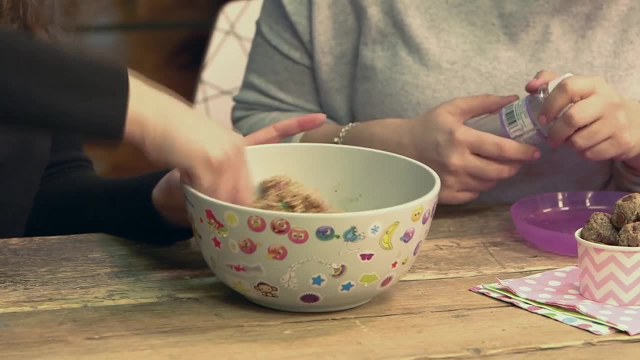 they don't fall off. Yeah, they don't feel cheated when they bite in. There's no sprinkle. Okay, I hadn't thought of that Like that. That's good. Definitely more fun as well. Look at that. That looks so sweet. 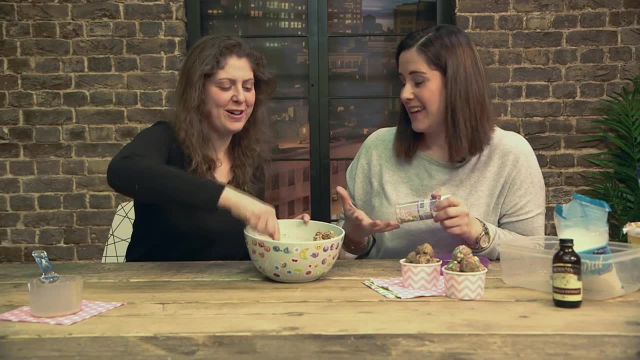 doesn't it Look at that? I love it. I'm excited It looks like cake And I'm not fine. You know I've got lots of kids who watch my channel, Thank you, So it's really nice to have. 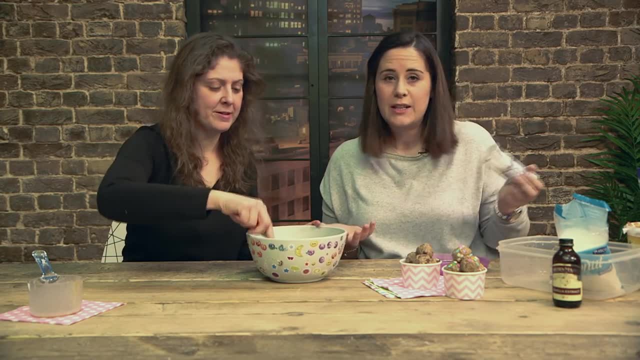 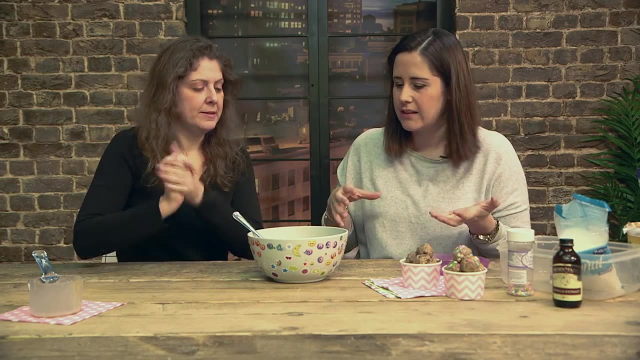 some fun things for them to make in the kitchen. It's great It is, And it's so easy because you don't need to cook, You don't need to turn on the cooker, You don't need to turn on the gas and the stove. It's safe as well, You know. you can leave the kids in the kitchen doing this. 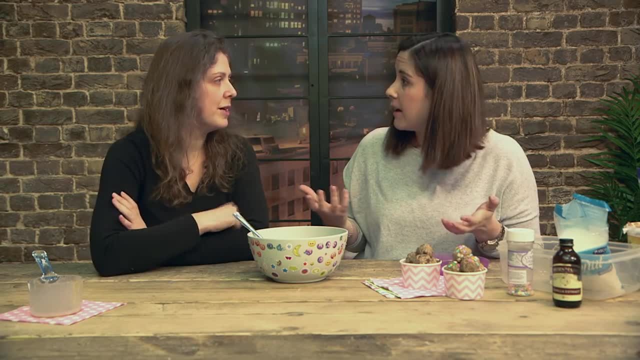 In the classroom, because I know they often make bakes at school. So that would be quite nice At school as well, wouldn't it? Absolutely Again. and it's really easy, And it's simple ingredients. I mean, I always have these ingredients at home. It's one of those. 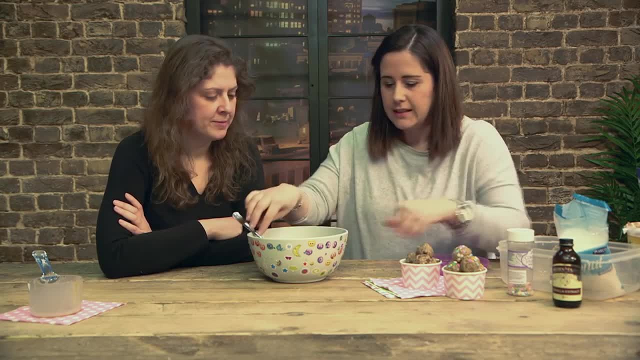 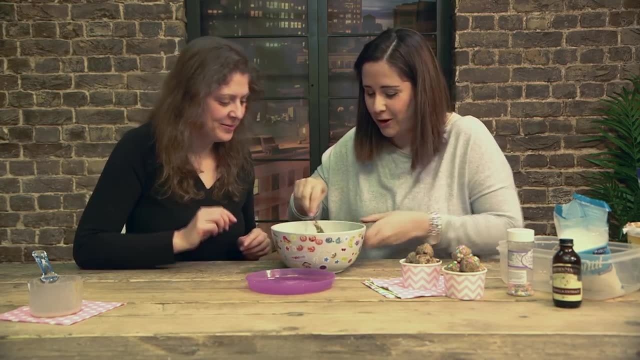 healthy store cupboard essentials. So yeah, And now we just roll, We just roll. You've done a great job, Yeah, really good, Yeah, So we're just going to roll If you want to just dig in, I mean. 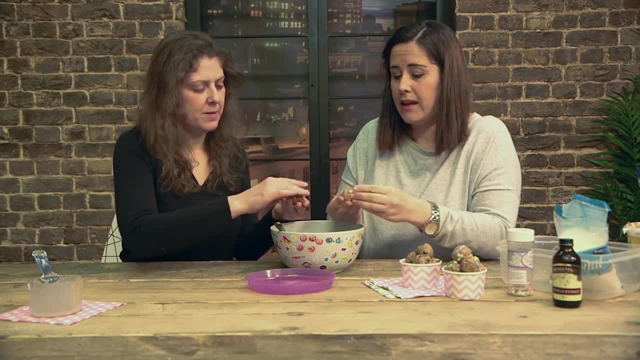 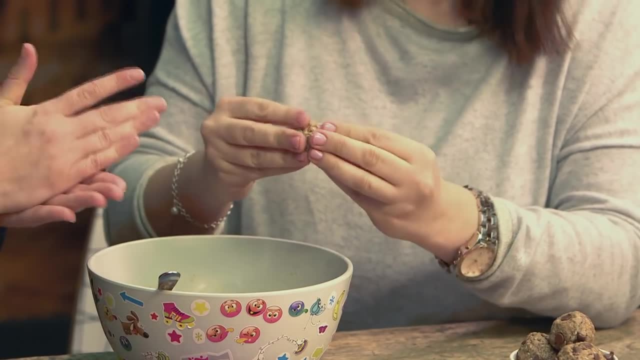 again, it just depends the size, the kind of bites you want to make. These are kind of generally the ones I make because my kids are a bit younger. Yeah, But for older kids I'm also thinking these would be good for. my kids often get an extra snack if they've got an afternoon club at school. 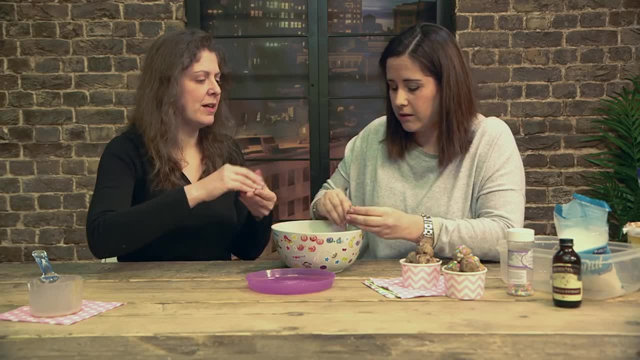 Yeah, So this is just to keep them going And also, we're not obviously nut-free school. We don't take, I can't take, give them. But this is nice bit of if I do it with the sunflower. 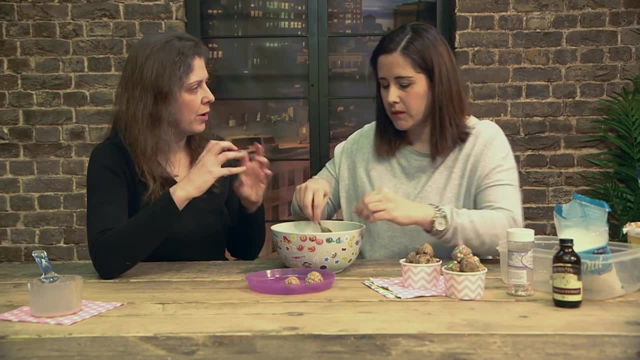 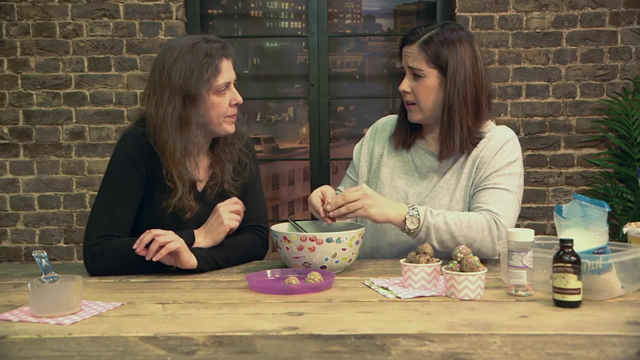 butter again Brilliant. And you say you refrigerate them just to hold them a little bit. Yeah, So we're just going to roll them up and then refrigerate, because you can see, the mixture is still quite soft. So if you refrigerate, probably for about anything from 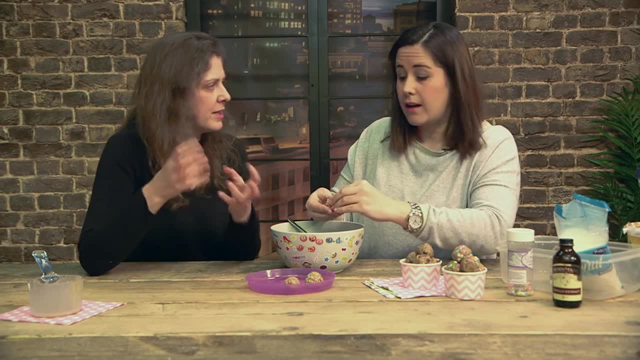 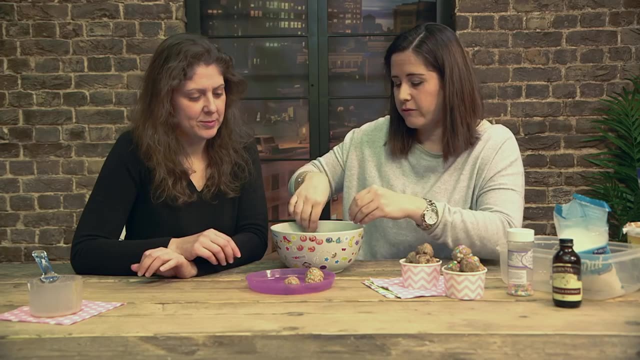 30 minutes, Okay, great, And they'll last the day after that as well. They'll last for several days, Okay. I usually make double, even a triple batch, And then I keep them in the fridge for I mean. 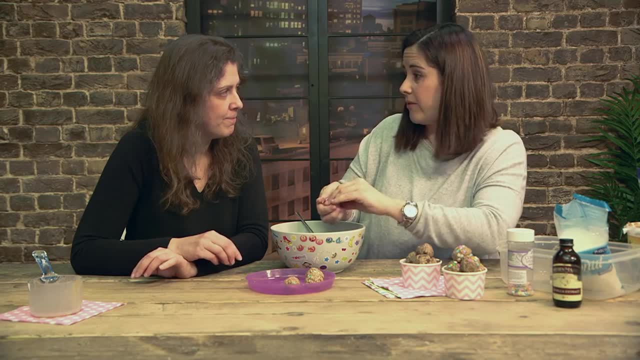 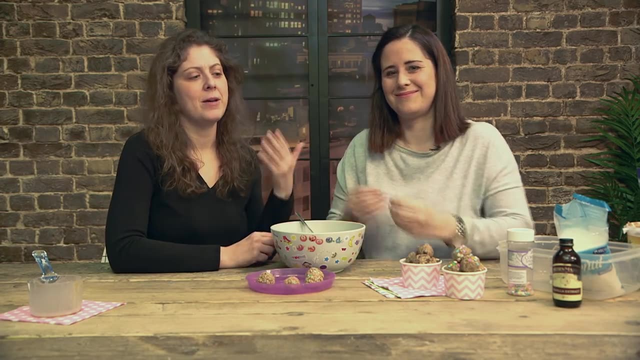 three to four days is absolutely fine. I usually keep them up to five. Brilliant, Excellent. So you've shown us how to make this. Stay tuned, because you must hear more about Ciara's channel and we'll talk all about it, And also make sure you visit, obviously. 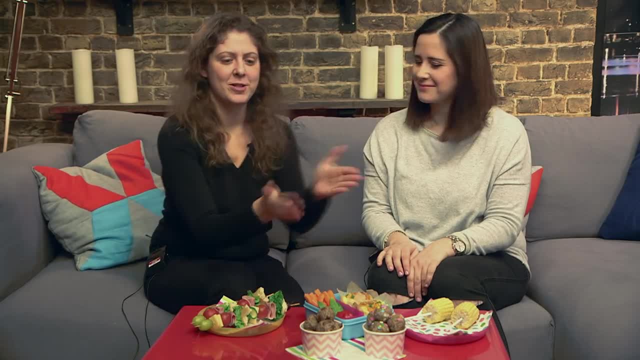 Right. So thanks for showing us how to make those Really yummy. So you can see our finished products. So show us what else you've got And tell us about the channel. Yes, So I've bought a kind of a selection of. 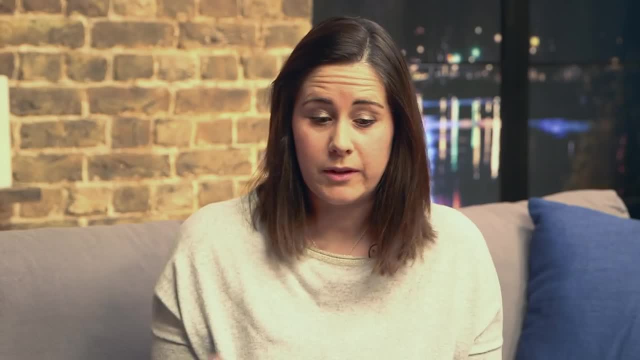 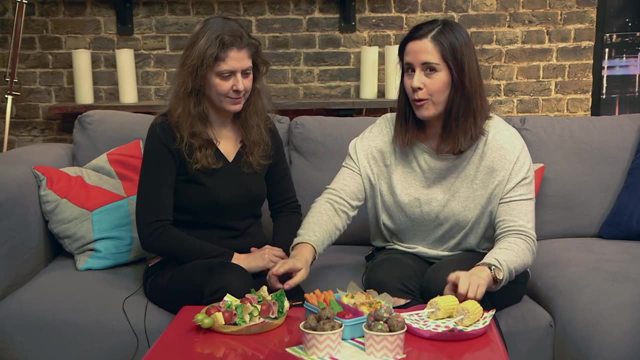 the kind of foods that I make. So, and it is basically the food that I make for my family, that I make for my kids. I'll start with these two first and explain why they are both on sticks. I have learned because I've got- my oldest child is four, going on five. I've learned over the last. 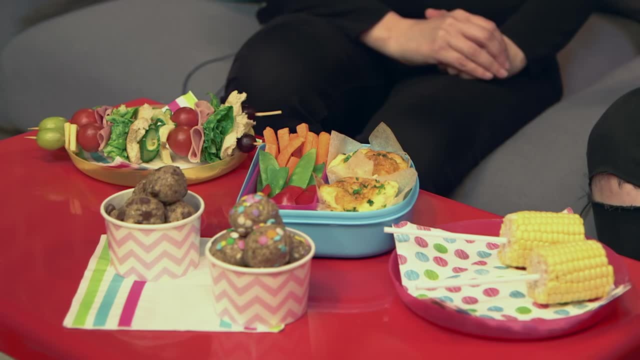 couple of years that if I put something on a stick, she's more inclined to eat it. It's funny, isn't it? I guess it's fun then, isn't it It is, And so many, so many parents have said the same. 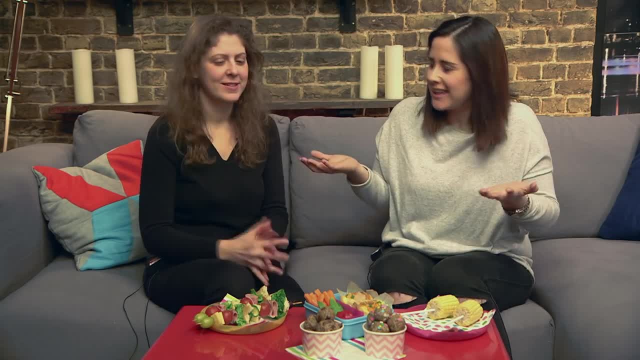 thing to me, since: How funny. So put a grape on a stick and they'll eat it. Just put it on a stick and they'll eat it. I love that Great idea. So, first of all, this is just such a simple idea, It's just basic. 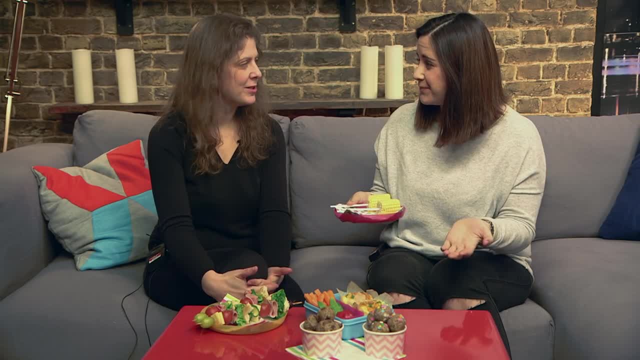 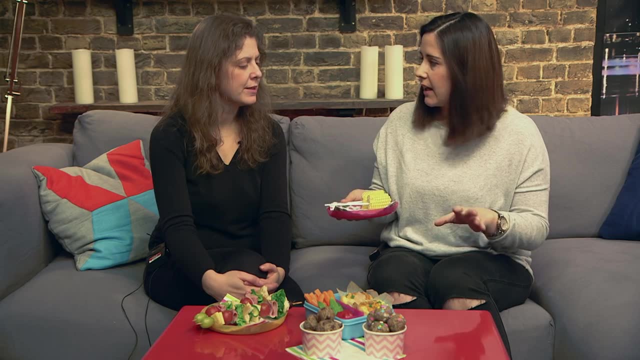 corn on the cob but on cake pop sticks And then instantly they want to eat it And they love it. I mean, my kids eat these for snacks now. So I sometimes boil them up, I keep them in the fridge and just I leave them out And it keeps those munchies under control. 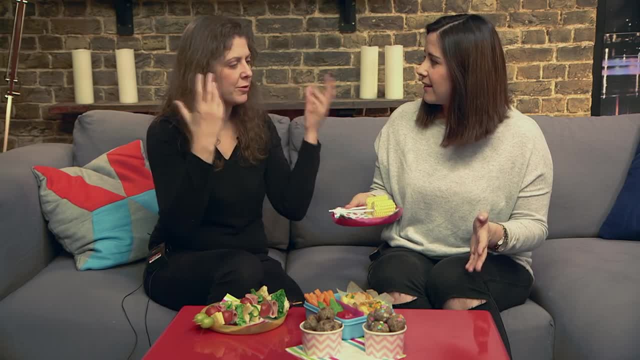 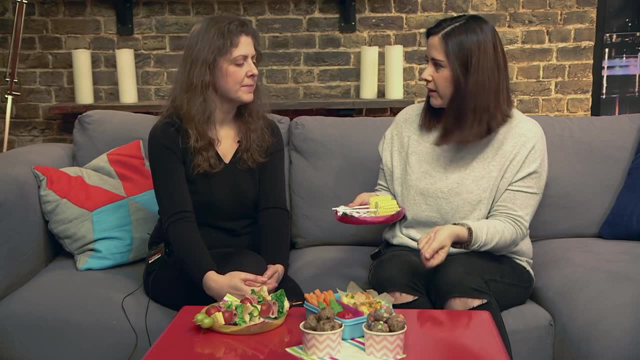 because they're kind of munching on it, rather than you know. sometimes you eat because you're bored, Exactly, Or that you know, like the kind of 10, 15 minutes before dinner is ready, the kids are screaming for food. Yes, Pop, one of these. 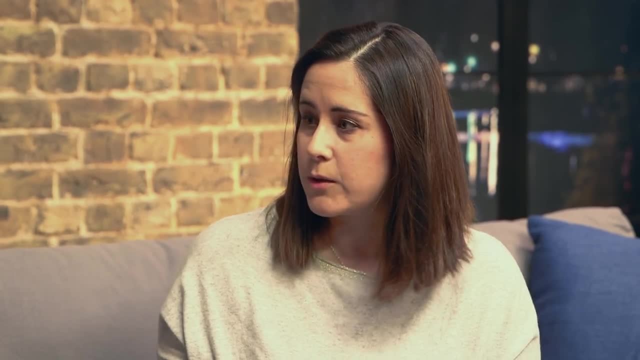 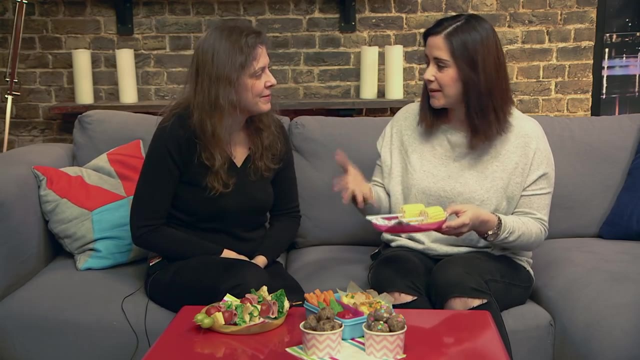 out from the fridge. If you want, just heat it in the microwave. A bit of butter, a bit of salt if they like that, And your candle is full of these genius little ideas that make life easier. It's just the little things to keep the kids happy and also to get some healthy food in them. 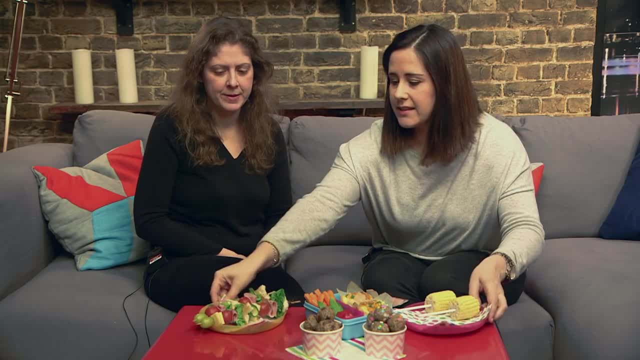 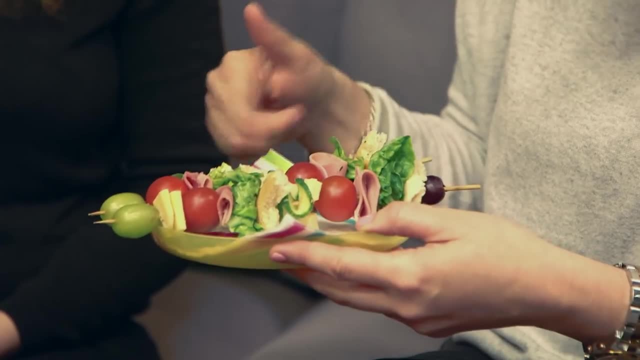 Brilliant, Simple ideas are always the best. Yes, I agree, I agree, And this again, another idea on a stick. but it's just, it's basically a deconstructed sandwich. Oh, of course it is. Yeah, So it's a ham and cheese sandwich with some lettuce? Yes, But it's. 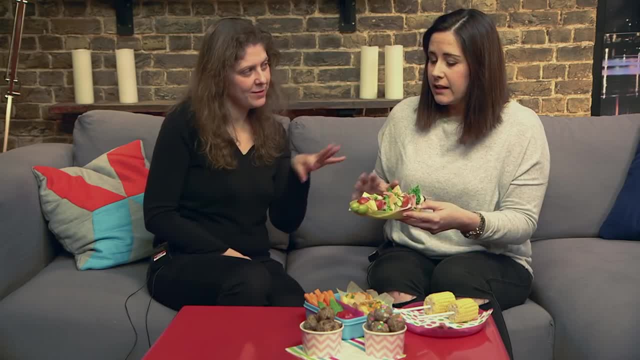 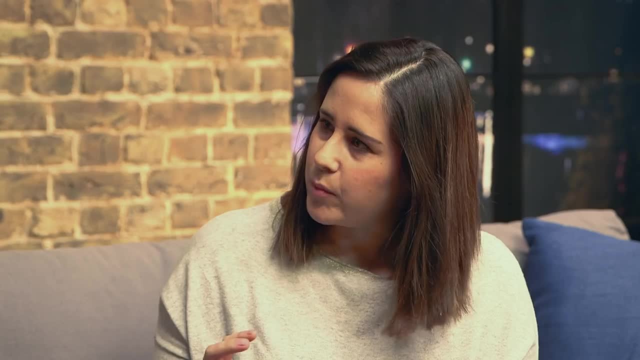 put on a stick And do you find they eat all of it or maybe leave the old one? There is things like things like lettuce. My daughter in particular doesn't really like lettuce, but when I serve it like this she'd have a little nibble, And that's what it's about. 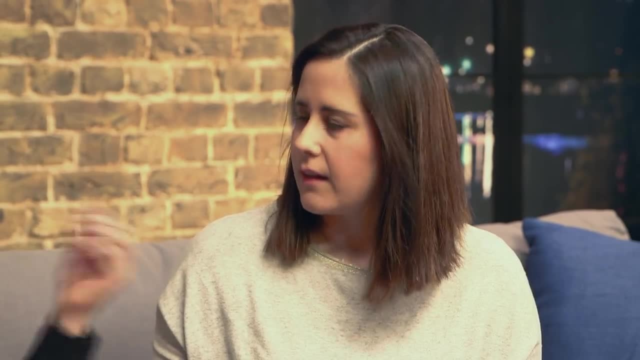 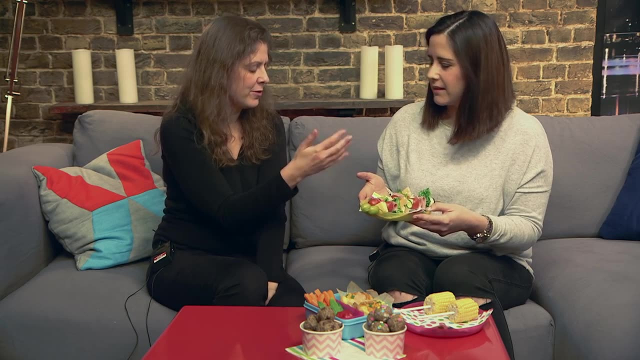 isn't it? It's just constantly introducing and constantly getting them to try, Because I find, for example with lettuce, that I've been really lazy about giving it to my children, But actually one of them does eat it, and it's because every so often I've remembered. 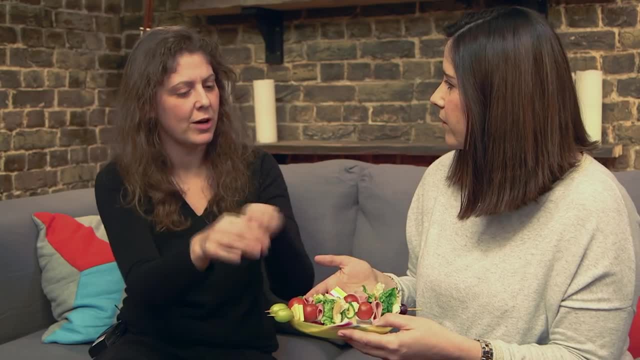 and it's that habit forming, isn't it? It is. So I guess this is really good, even if they don't eat all of it. you're habit forming and they're used to seeing it and I guess, nibbling it and tasting it It is. And there's all this. 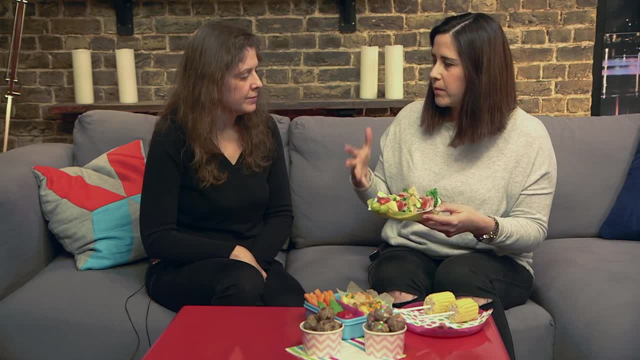 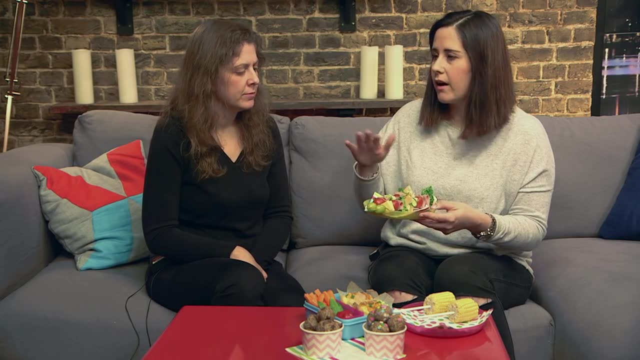 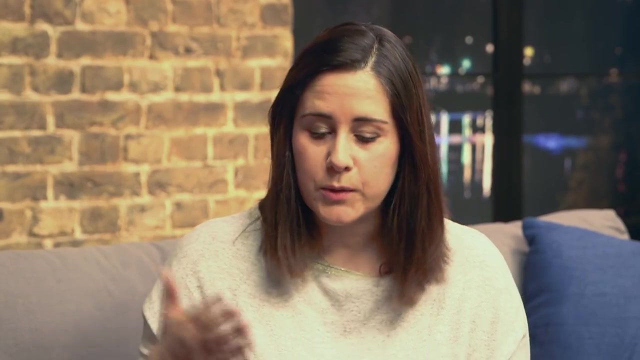 research at the moment about kids' feeding habits and how to introduce new foods, And it's all about just small tastes, small bites, small tastes, And even if they say I don't like that, try it again in a couple of weeks time because their taste buds expand and develop so quickly. So it's always 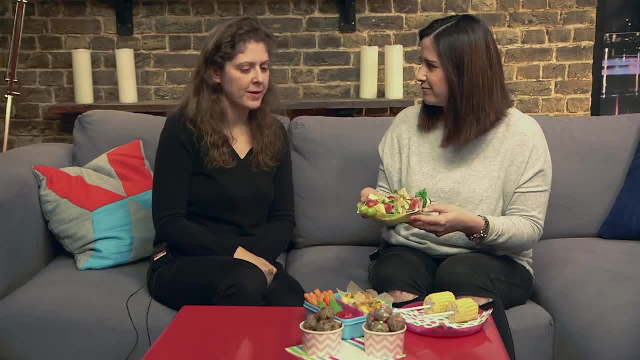 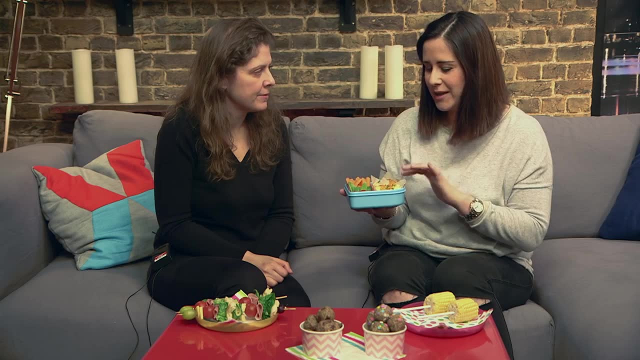 worth trying. If they don't eat it this week, try next week and the week after. Let's see these. These are probably one of my favourite recipes to make, because I basically serve them all day long. They're excellent. They're excellent. 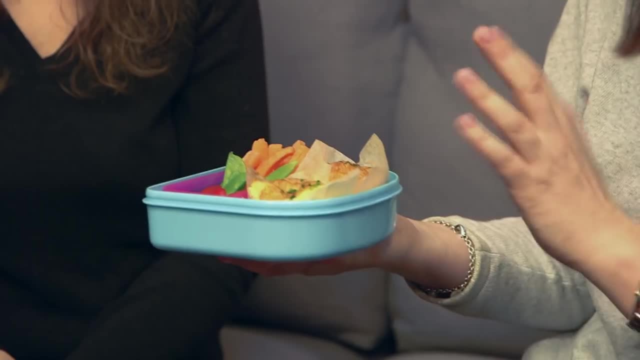 Muffins. they can be breakfast, they can be lunch, they can be a snack, they can be tea. They're quick to make, They are. They take about 20, 25 minutes in the oven. Okay, that's right. Yeah, yeah. 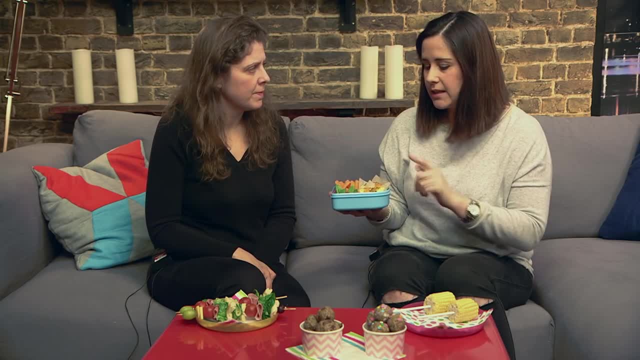 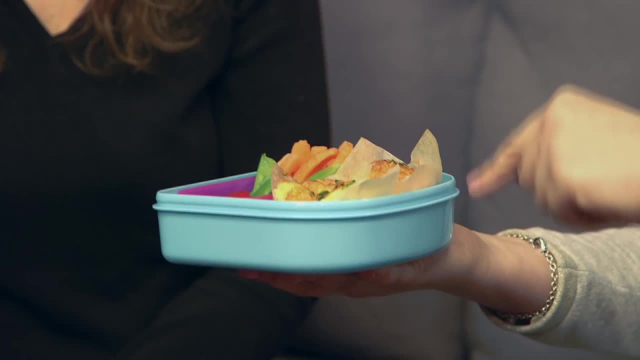 But in terms of preparation they are so simple, Brilliant. So all you need is some eggs. So say you want to make six, you need six large eggs, chuck in and beat them up in a jug, chuck in some grated cheese and then any extras. So 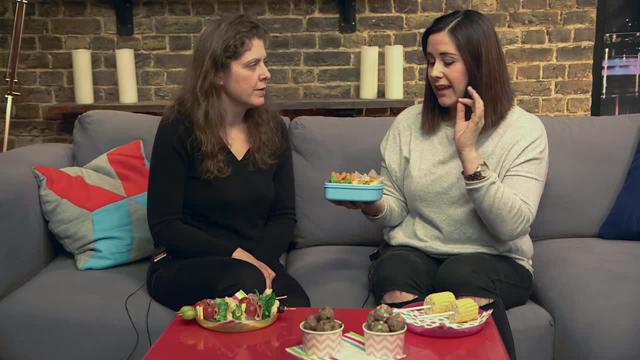 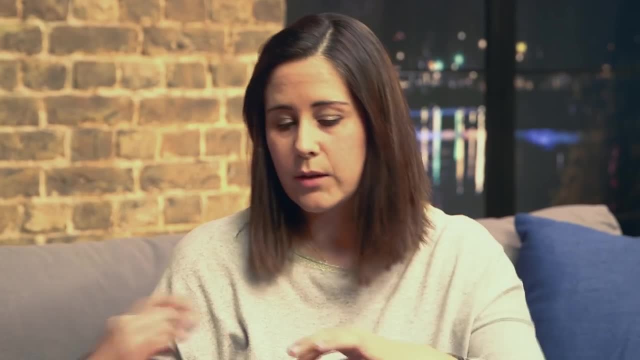 you can put in like ham cooked chicken. again, secret little veggies, chopped up veggies. pour them into muffin tins. Yes, with the paper. Yeah, so a little bit of paper. You don't even have to If you use the silicone. 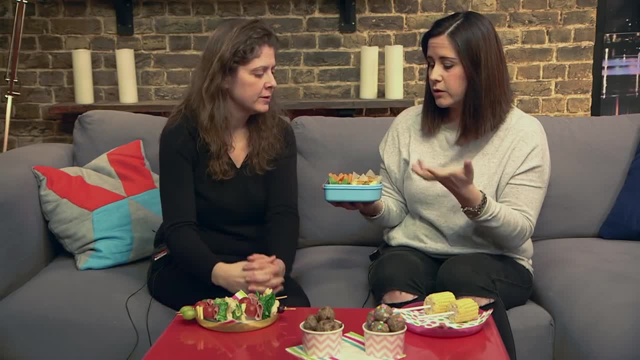 Oh, it'll come out. Yeah, they'll pop straight out. Brilliant, yeah. Put them in the oven 20, 25 minutes and they're ready. Brilliant, yeah, You can eat them warm straight away. keep them in the fridge for a couple of days.